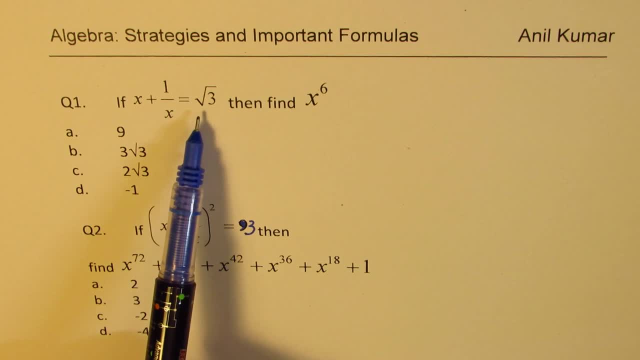 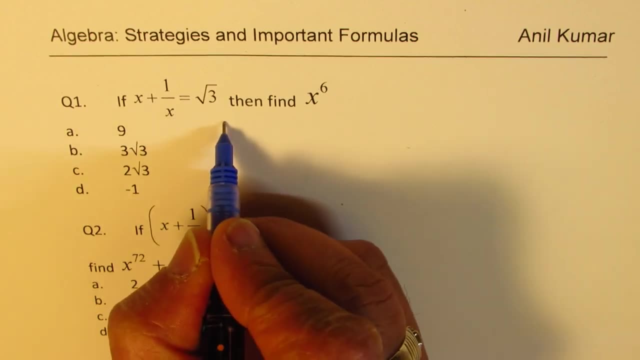 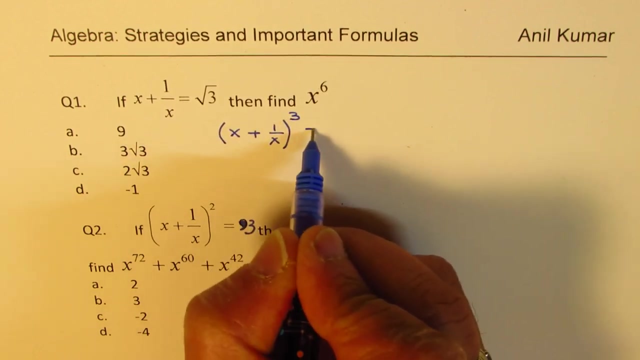 when we find the value of x to the power of 6. We are given x plus 1 over x equals to square root of 3.. Okay, so what we are going to do here is, to begin with, we will do cube of x plus 1 over x, right? So we will do cube of this. So I hope you. 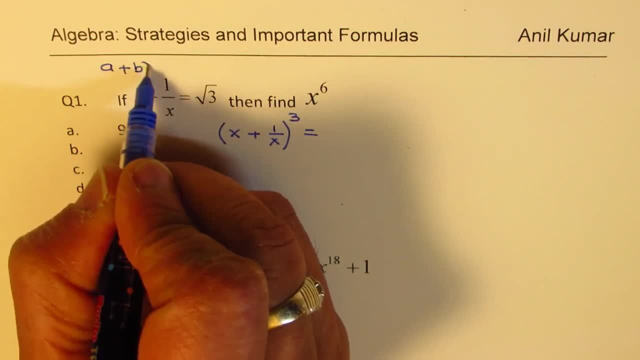 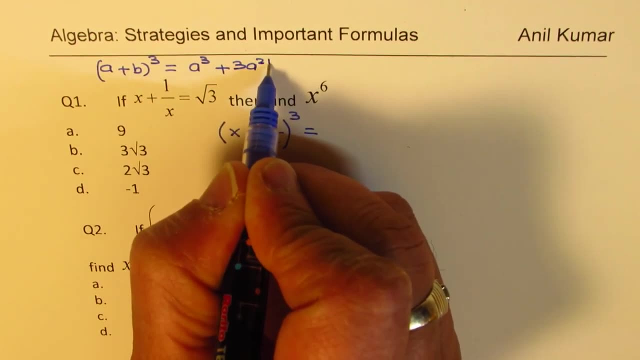 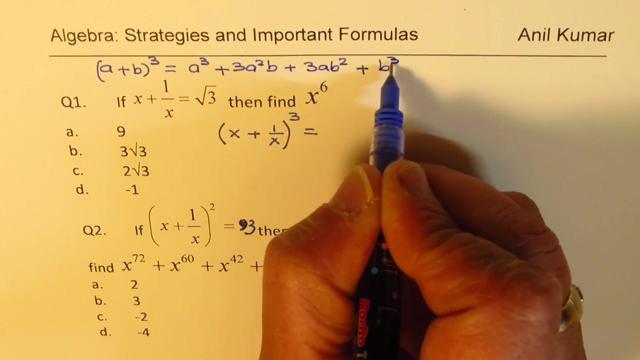 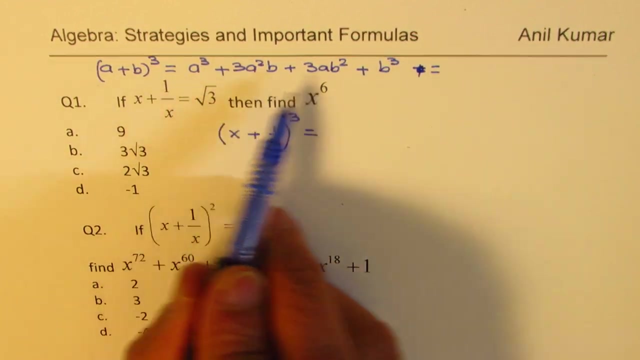 remember the formula for the cube which is a plus b whole cube is equal to a cube plus 3 a square b, 3ab square plus b cube. right Now you could actually rewrite this formula in kind of a factored form rearranging. We could write this as a cube plus b cube right And the terms in 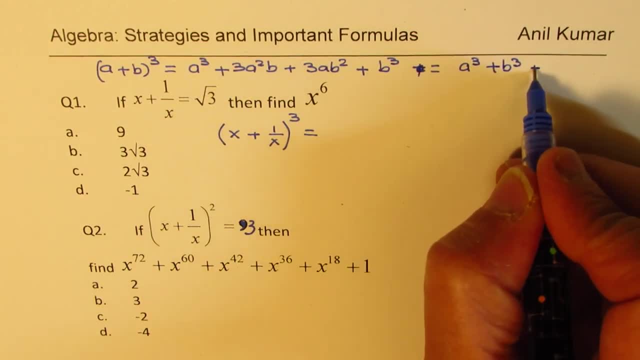 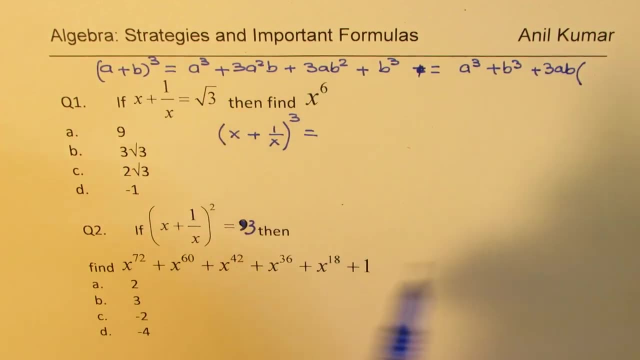 between are: 3ab is common, so we'll say plus 3ab. So if you take 3ab common, you get a plus b, right? So a plus b. Does it make sense to you? So that is how you could actually write the. 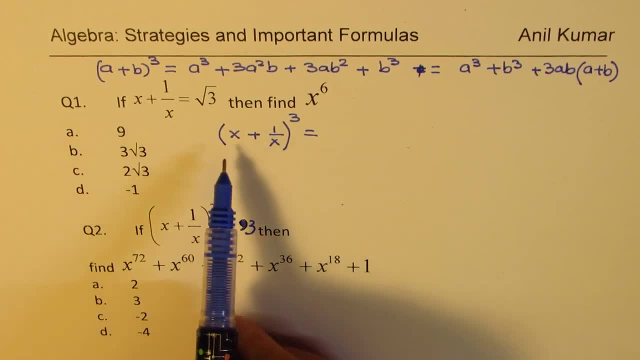 formula for a plus b: whole cube. So we are given x plus 1 over x as square root of 3. We'll just cube this and rewrite. So x plus 1 over x is to the power of 3.. So when we cube, what do we get? 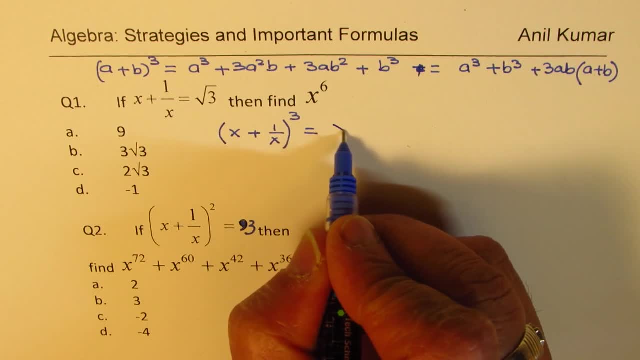 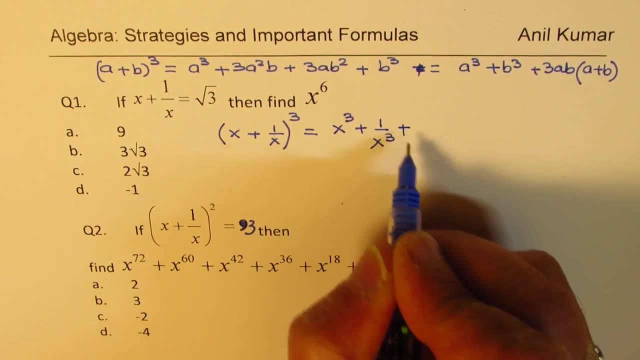 We'll apply this formula right. So a cube plus b cube, So cube of x will be x cube plus cube of 1 over x will be 1 over x cube plus 3 times ab. That means 3 times x times 1 over x. 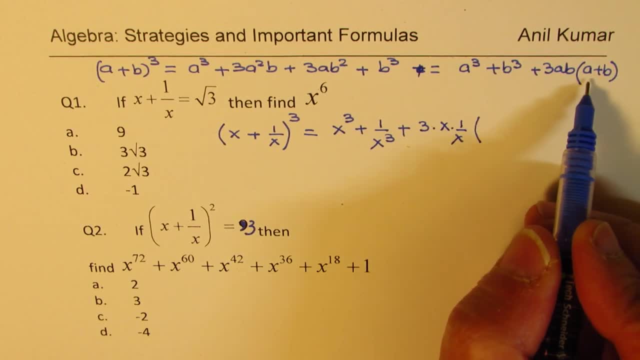 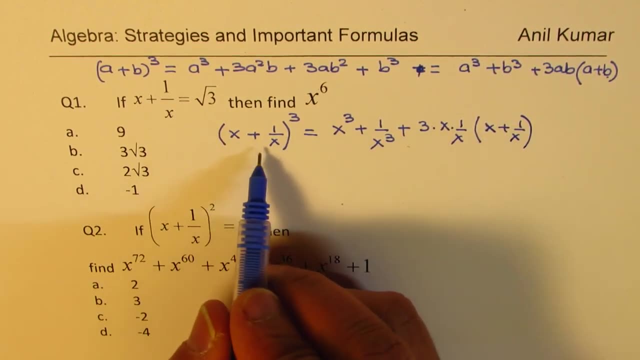 And within the brackets, you get x plus 1 over x, which is sum of a and b, right? So we get x plus 1 over x, correct? Now we know that x plus 1 over x is equal to square root of 3.. So 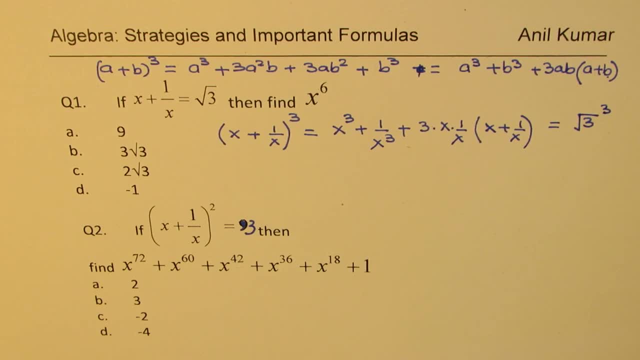 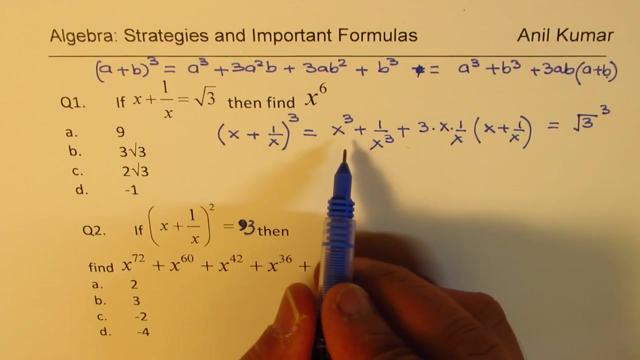 we'll kind of cube this. So that is how we will begin Now in this. what you really see is that x cube plus 1 over x cube can be written as equal to. let's rewrite this So from here. what we get here is that x cube. 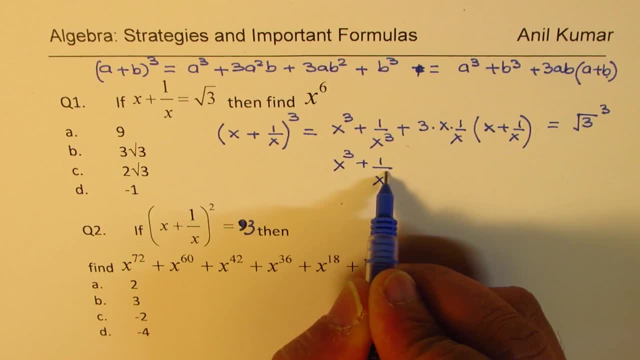 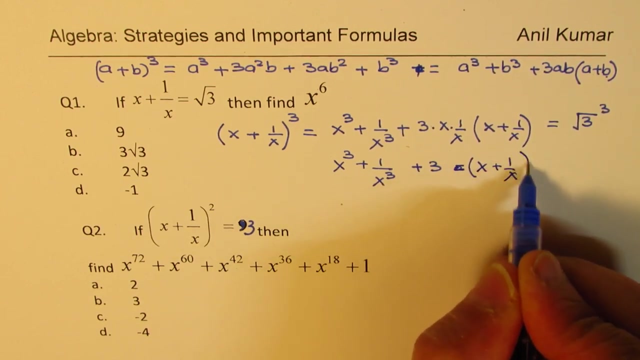 plus 1 over x cube. x over x cancels right. So plus 3 is equal to sorry. in the bracket we have x plus 1 over x. right is equal to 3 times square root of 3, right. 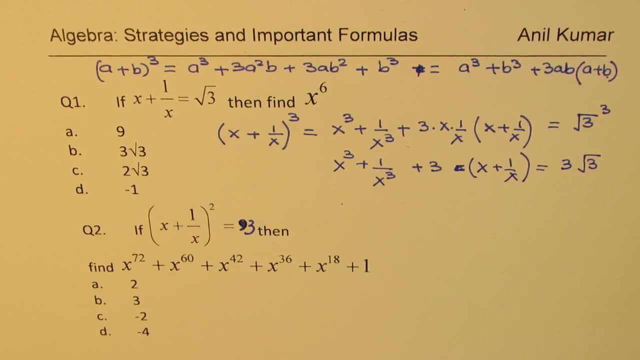 So when you cube this, that is what you are going to get. Now we know what is the value of x plus 1 over x. It is square root of 3.. So we could write this as x cube plus 1 over x cube plus 3. 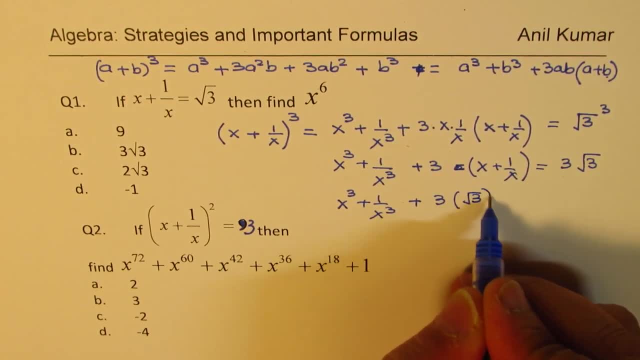 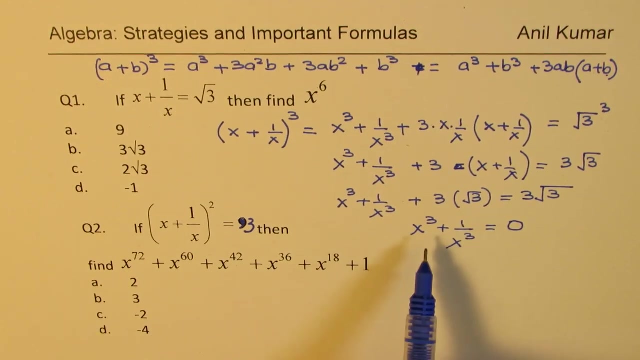 times This is square root of 3, equals to 3 times square root of 3.. Now that really means that x cube plus 1 over x cube should be equal to this minus this, which is 0.. To solve this equation: 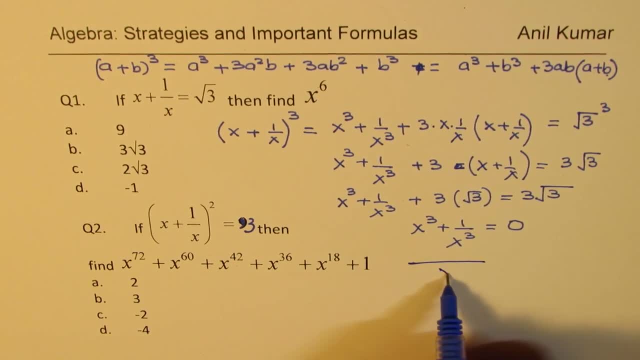 we could take x cube as a common denominator, right? So if I take x cube as a common denominator, I get here: x to the power of 6 plus 1 equals to 0. Now, denominator cannot be 0. That means 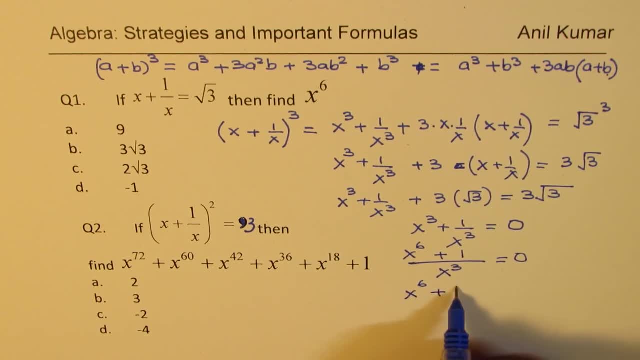 means x to the power of 6 is or plus 1 is equal to 0,, or x to the power of 6 is equal to minus 1.. So we get the result for x to the power of 6.. So from here what we learn? 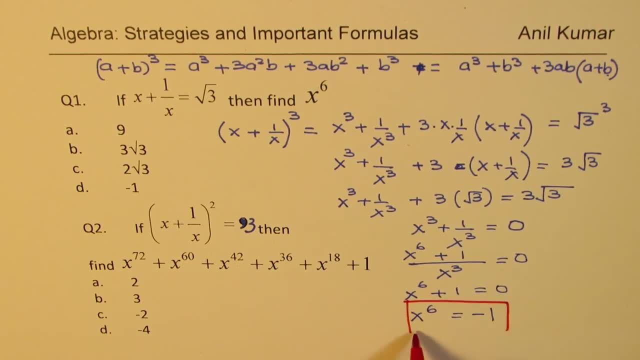 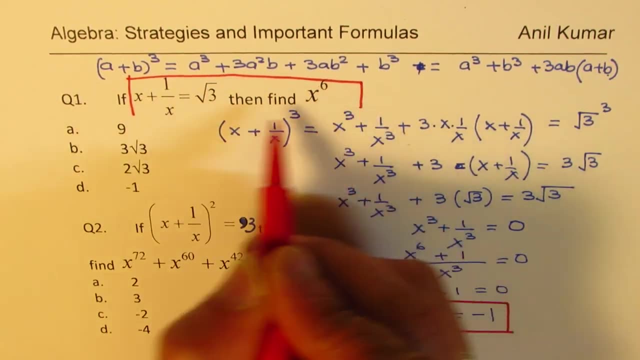 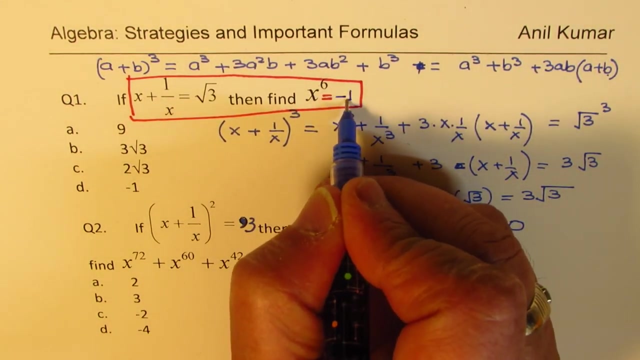 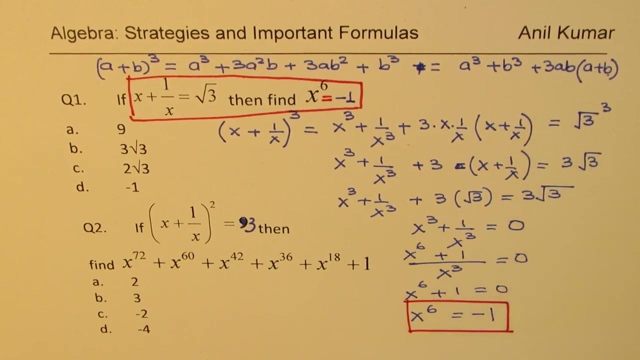 is that if we are given that x plus 1 over x is square root of 3, in that case x to the power of 6 is equal to minus 1.. Perfect. So that is a very important result which we have got here right. So that is the derivation for this particular result. Now, once we have 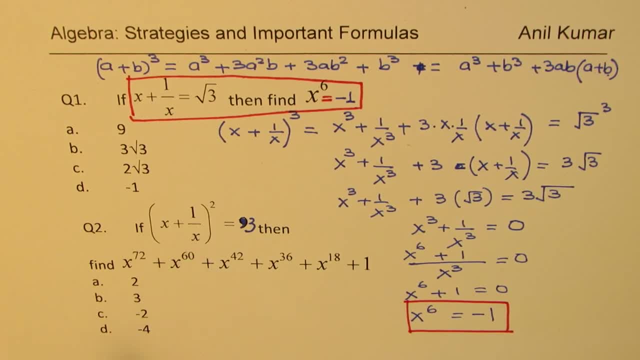 got this, then let's try to understand how to solve the given question Now. in question number 2, we are given that if x plus 1 over x square is 3, that really means that really means that x to the power of 6 is equal to minus 1.. So that is the derivation for this. 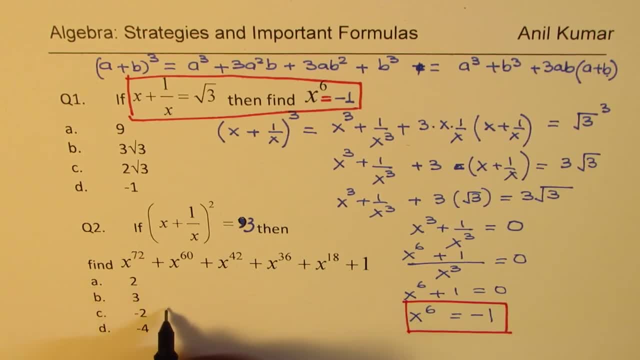 case. So that means that what we are given here is: x plus 1 over x is equal to square root of 3.. Now, if that is the case, in that case we know that x to the power of 6 is equal to minus 1, which we have just derived Correct. Now we could use this result to solve. 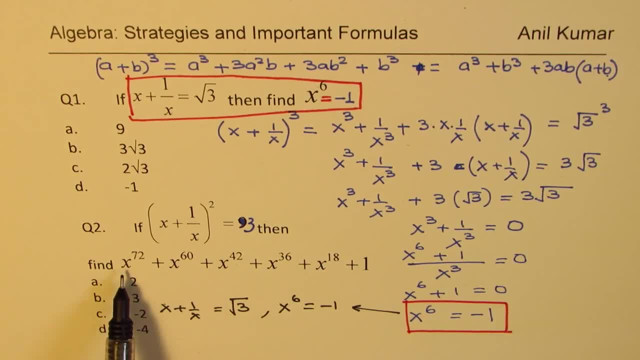 such expressions. Now, when I say x to the power of 72,, 72 is a multiple of 6,. 60 is also a multiple of 6.. 42 is 6 times 7,, 36 is 6 times 6,, 18 is 6 times 3, and the number 1.. So what we could do now? 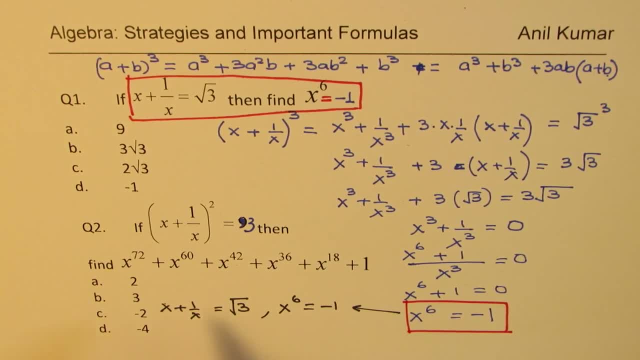 is: rewrite this expression as powers of 6.. So we could write this expression as x to the power of 6 to the power of 72 becomes 12.. Now here it is x to the power of 6 to the power of 10.. And this is x to the power of 6 to the power of 7.. 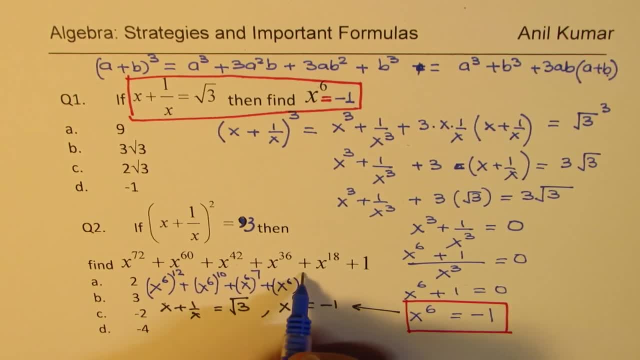 That gives you 42. Plus x to the power of 6 to the power of 6, and this is x to the power of 6 to the power of 3, plus 1.. Now, when you have even powers, since we know, this is x. 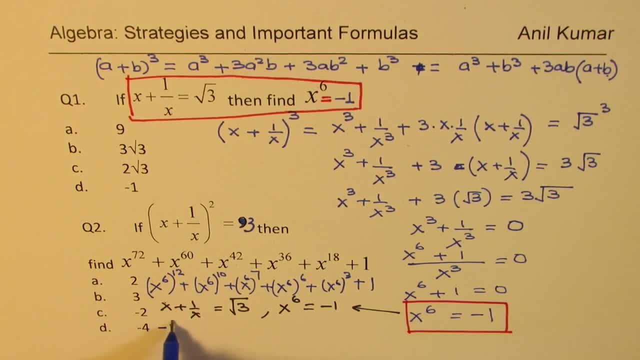 to the power of 6 is minus 1,. let me rewrite here: Minus 1 to the power of 12 plus minus 1. to the power of 10 plus minus 1. to the power of 7 plus minus 1. to the power of 6 plus minus. 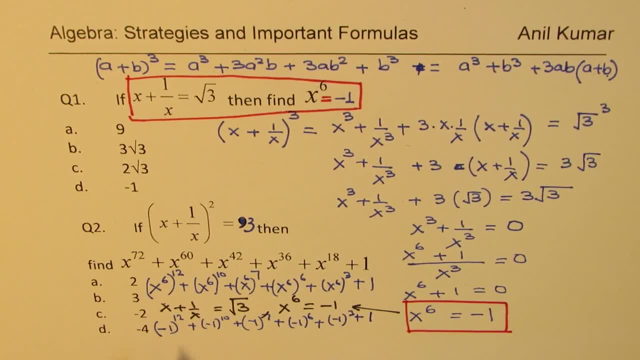 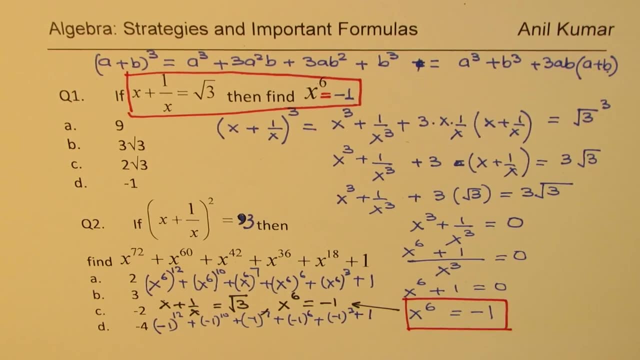 1 to the power of 3.. 3 plus 1.. All these powers, which are even, will result into positive 1.. So we get this as- let me push this a bit here. so we'll get this as 1.. Here again, we get positive 1.. 7 will result. 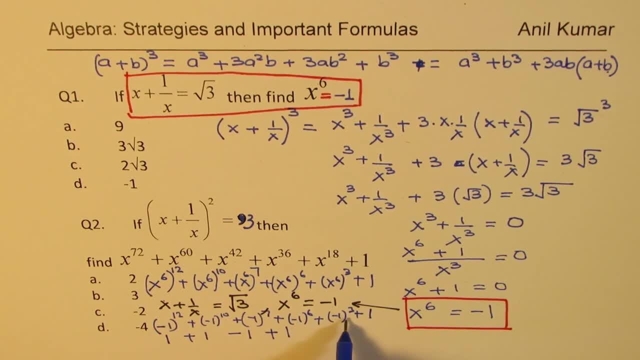 into negative 1.. 6 will result into positive 1 to the power of 3. negative 1, and then we already have 1 here. So what do you get? So there are two negatives, which kind of cancel it? So this cancels. 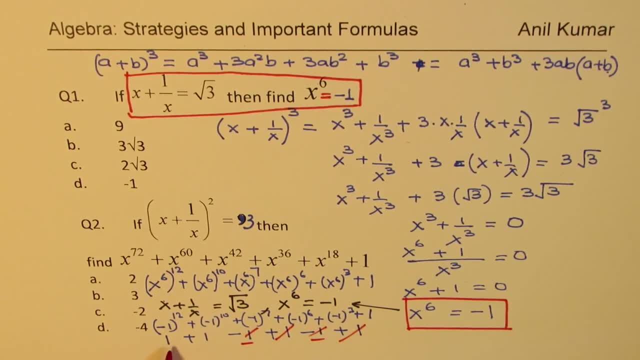 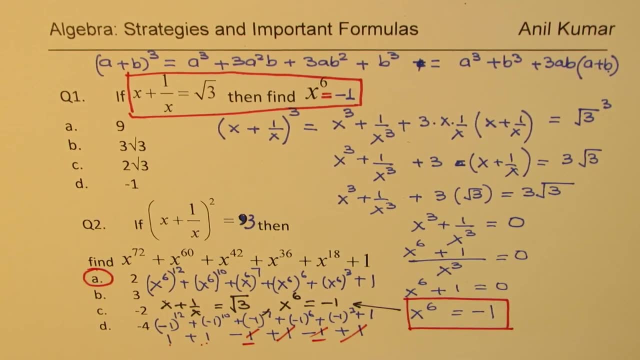 with this and this cancels with this right. So these cancel. We are left with 1 plus 1, which is 2.. So the answer is A for us. You get the idea. So that is how we could actually solve such a.